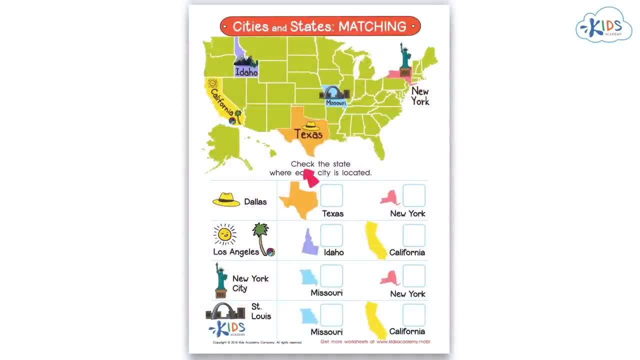 Read the directions. Check the state where each city is located. Look at the first row city. The name of this city is Dallas. Cowboy hats are popular in Dallas. Where is Dallas located? Yes, Dallas is a city in the state of Texas. Nice work. The next. 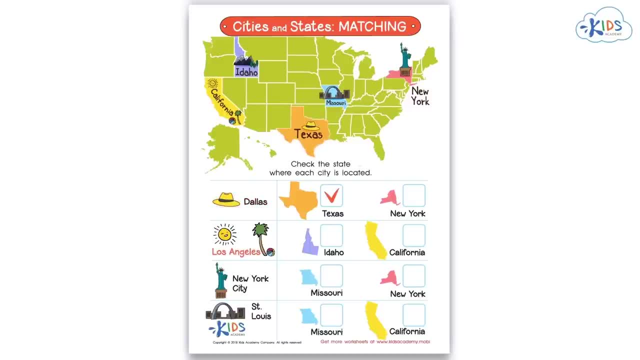 city is Los Angeles. Los Angeles is known for its sunny weather and beaches. Where can you find Los Angeles? That's right, Los Angeles is in the state of California. Great job. Now let's find New York City. You can see the Statue of Liberty when you visit New York City. Where is New York City located? 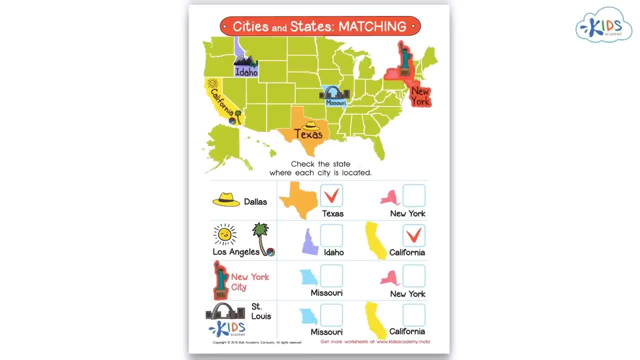 In the state of New York, of course, Good choice. The last city is St Louis. The Gateway Arch is a famous landmark in St Louis. In which state would you find St Louis? Missouri? That's correct, Congratulations. 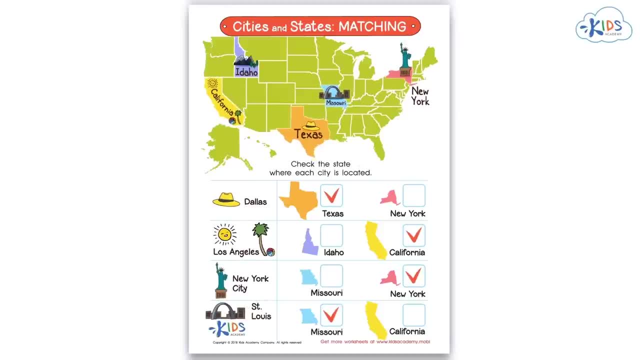 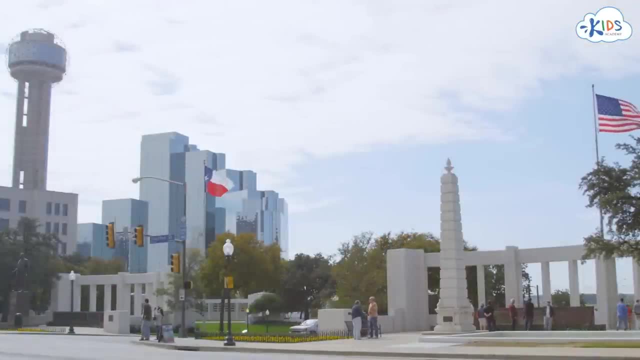 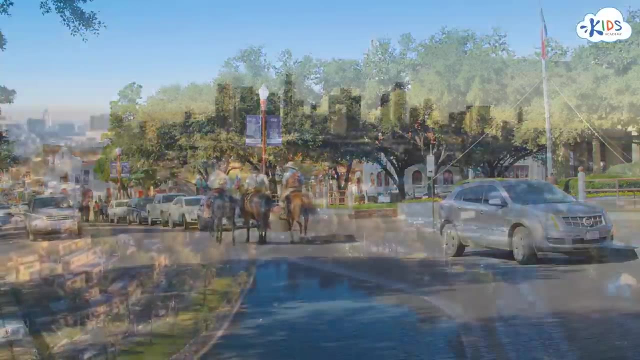 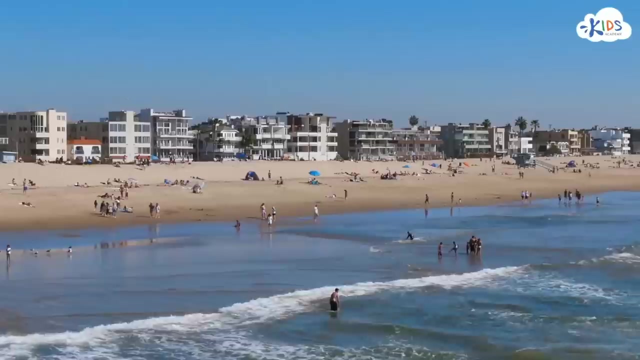 You've completed the worksheet- Awesome work. Let's review. The first city is Dallas. It is located in the state of Texas. Cowboy hats are popular in Dallas. This is Los Angeles. It's in the state of California. Los Angeles is known for its sunny weather and beaches. You can see the Statue of Liberty when you visit New York City. This city is located in the state of New York. The last city is St Louis. You would find it in the state of Missouri. The Gateway Arch is a famous landmark in St Louis. 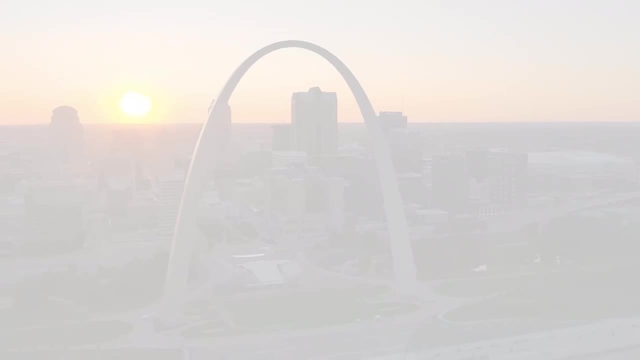 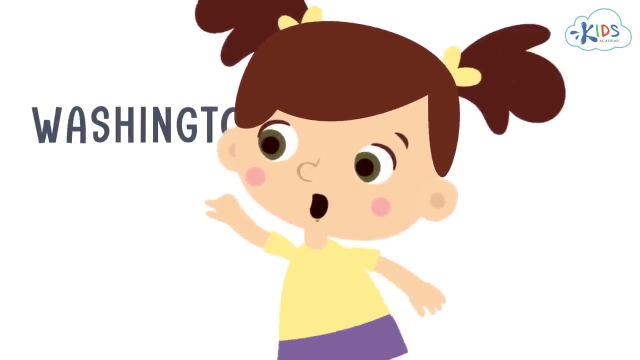 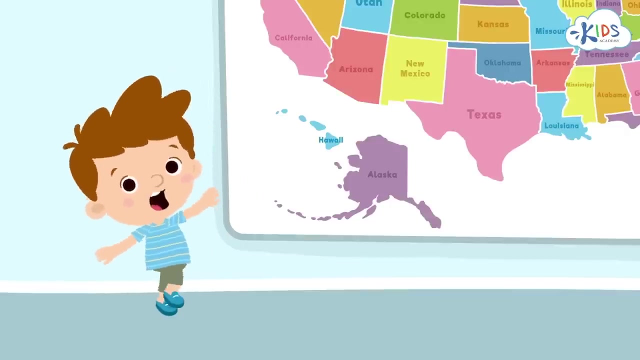 Thanks for watching. Goodbye. Hello, boys and girls. Today we are going to talk about Washington DC. Washington DC is the capital of the United States of America. I am so excited that we are flying there today. 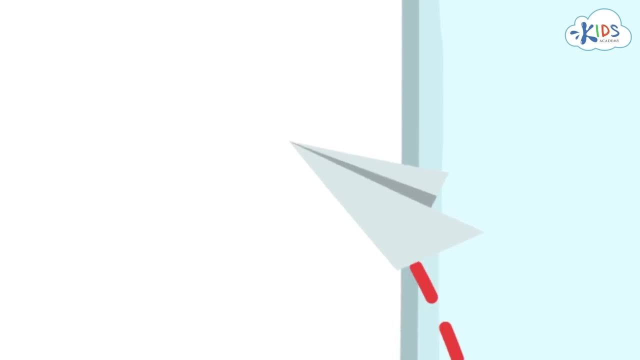 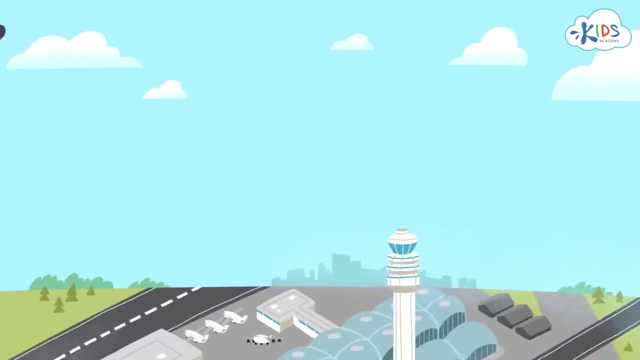 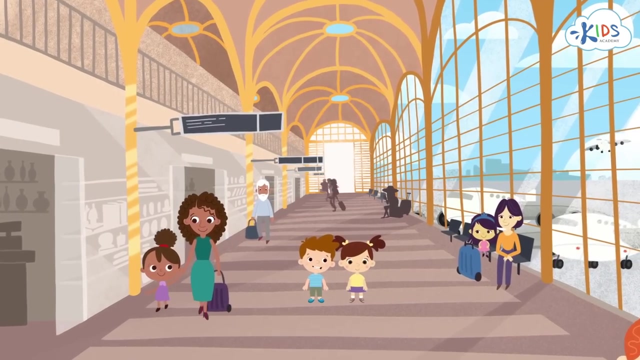 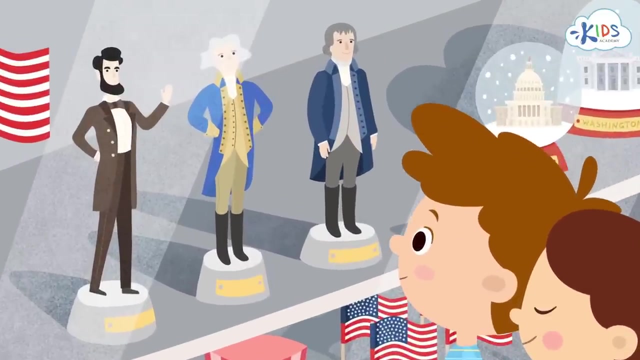 Me too. Let's go. Washington DC is the city where each US President lives and works. That's why you can see the Presidents, even at the airport. Well, not in person, of course, but there are portraits and statuettes. 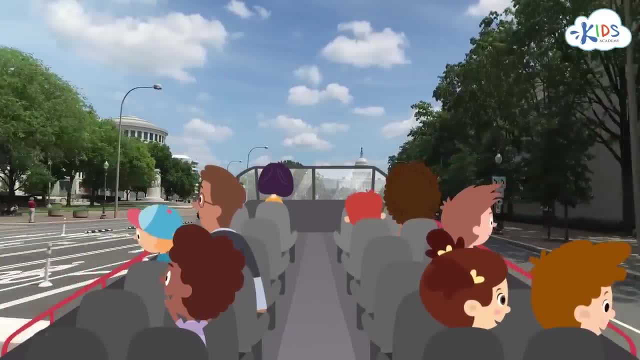 Washington DC is home to the United States of America. Washington DC is home to the United States of America. Washington DC is home to the United States of America. Washington DC is home to the US Government. 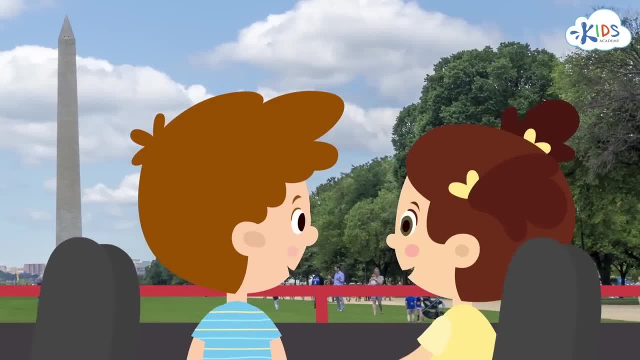 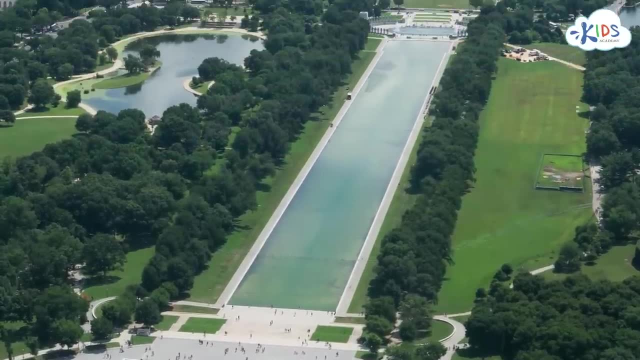 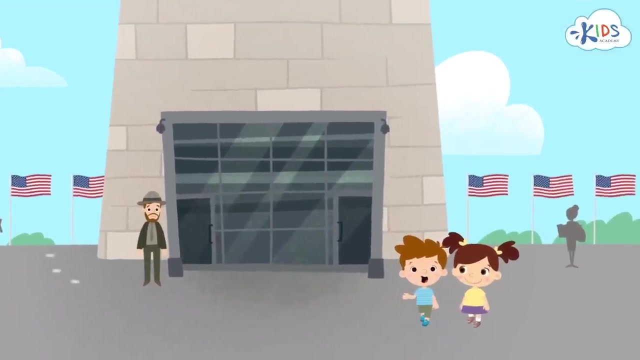 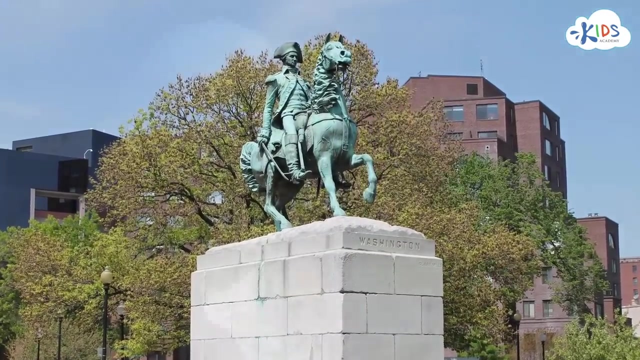 Many important laws and decisions are made here. Look, It's the National Mall. It is a large park with plenty of landmarks along its length. The city was named after George Washington, the first President of the United States. George Washington was one of the founders of the American government. 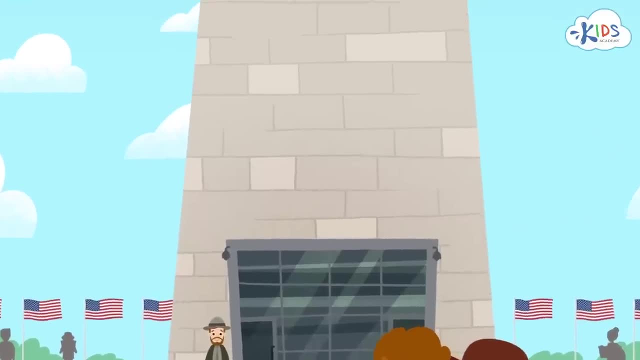 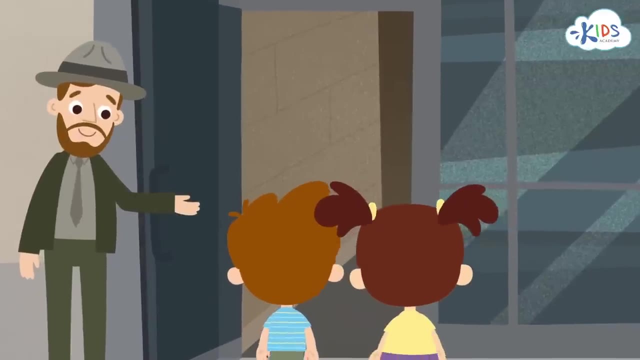 The city was named after George Washington, the first President of the United States. The Washington Monument was built in his honor. Wow, It's so tall. Yes, Let's go inside. If we go upstairs we can see the whole city. 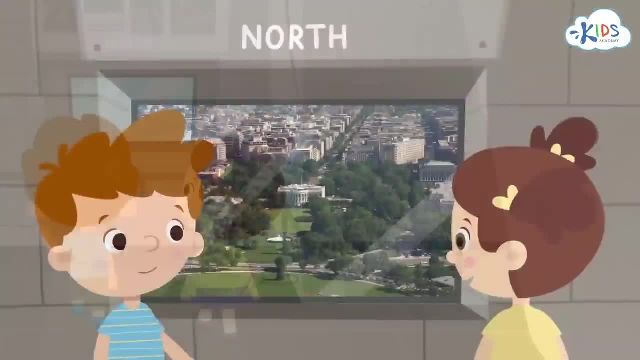 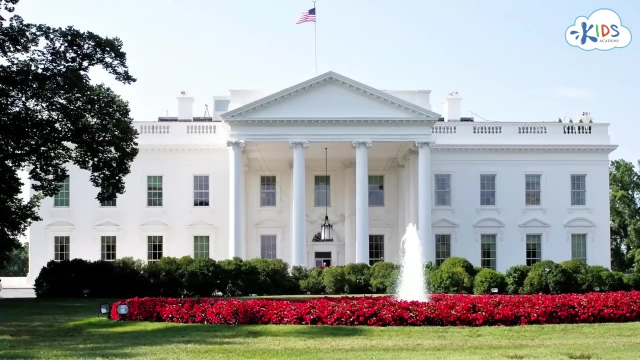 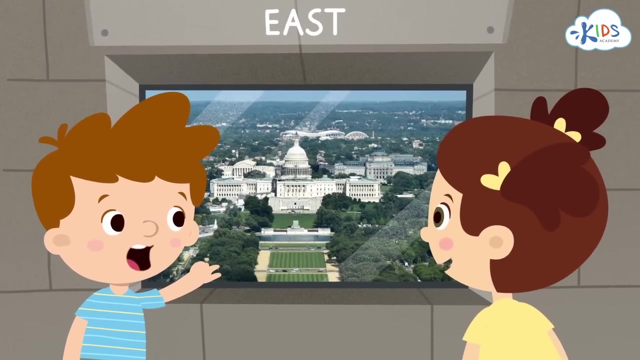 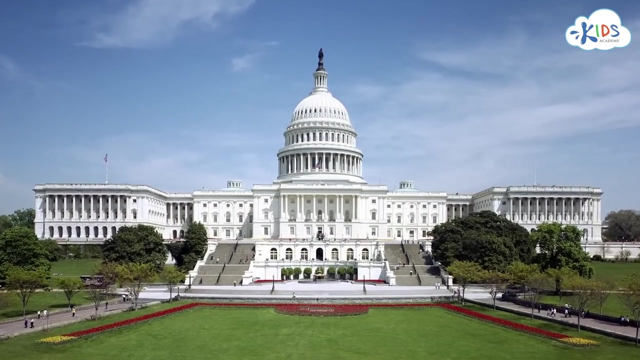 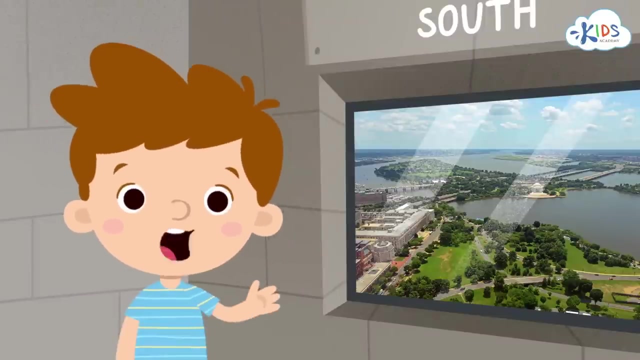 You can see more important places from here too. There's the White House. American Presidents live and work there, And this is the US Capitol Building. Congress leaders meet there to make important decisions about our country. To the south and west of the Washington Monument, there are two more memorials of famous American Presidents. 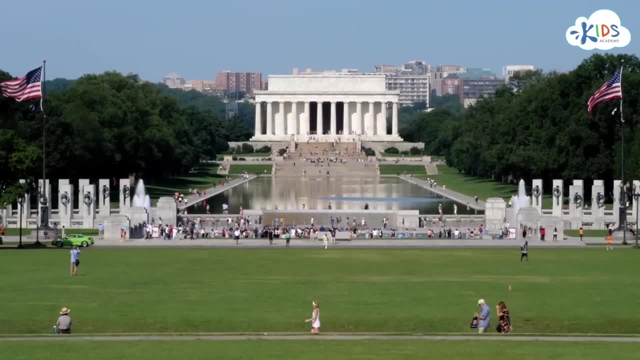 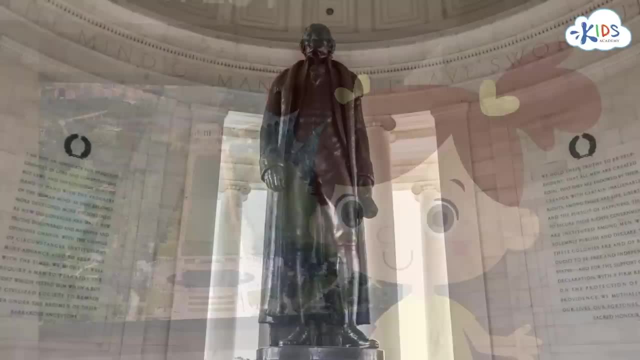 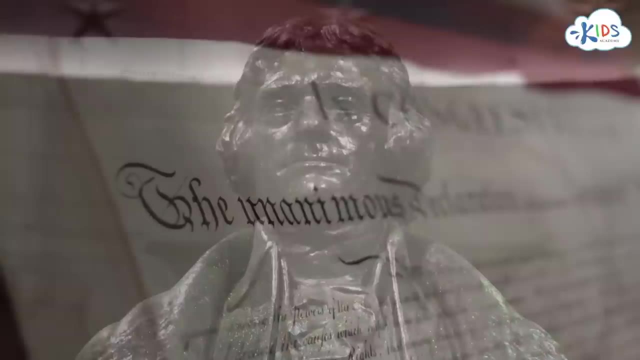 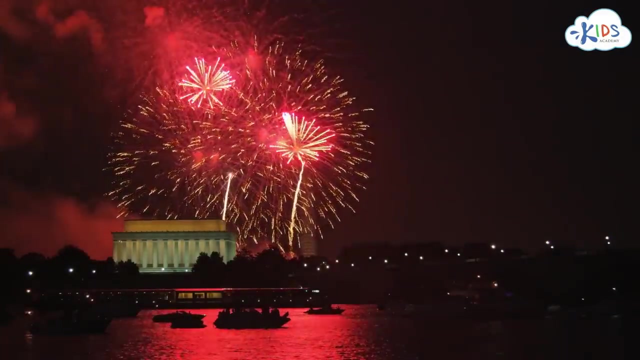 Thomas Jefferson and Abraham Lincoln. Oh, Tell me about them. Thomas Jefferson was one of the authors of the Declaration of Independence. The day it was adopted, the 4th of July, became one of the most important holidays in America. We call it Independence Day. 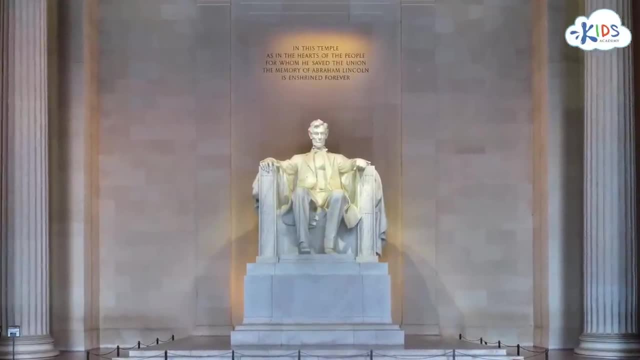 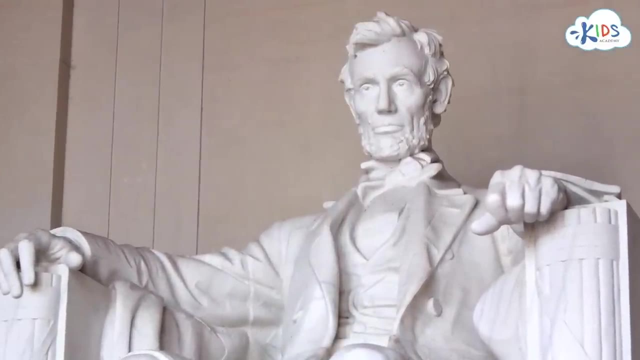 And what about Lincoln? Abraham Lincoln was the 16th President of the United States. He signed the Emancipation Proclamation. He signed the Emancipation Proclamation So that all Americans could be free from slavery. So that all Americans could be free from slavery. 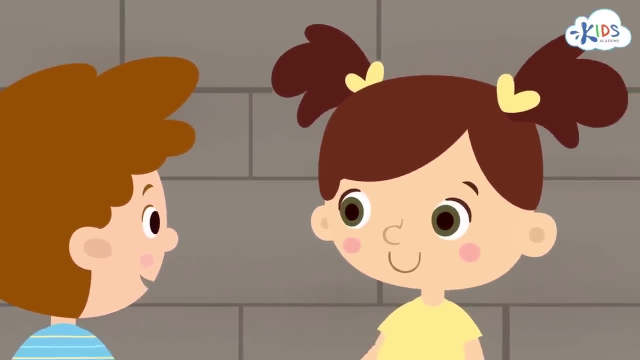 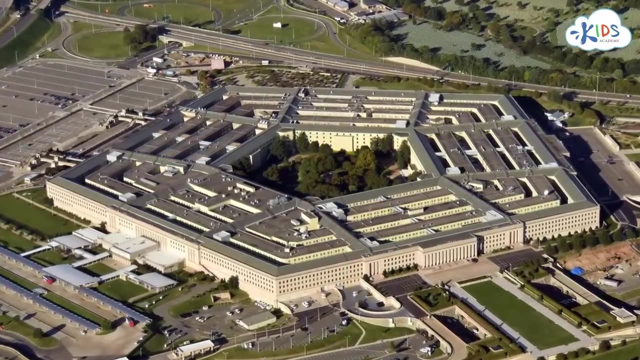 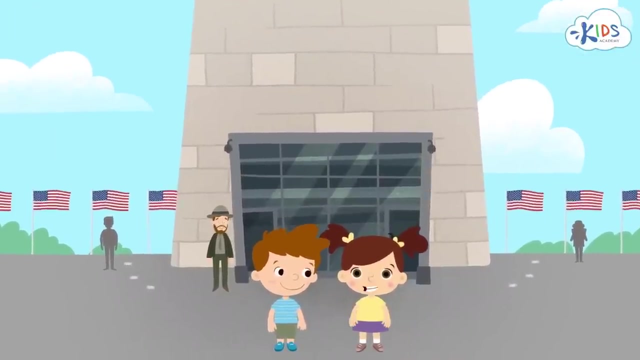 What else can we find in Washington DC? Lots more Like the Pentagon Building Where the US Department of Defense works. They work hard to keep our country safe. I love the shape of the Pentagon Building. Where should we go now to have some fun? 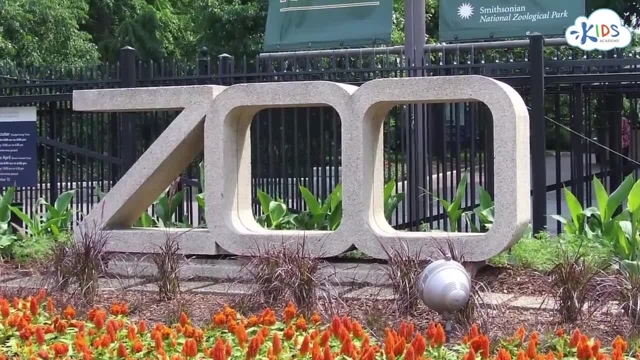 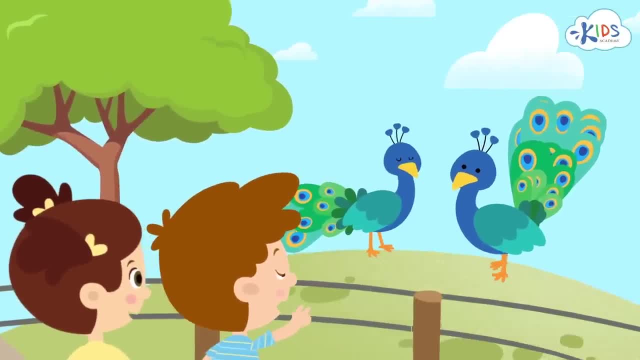 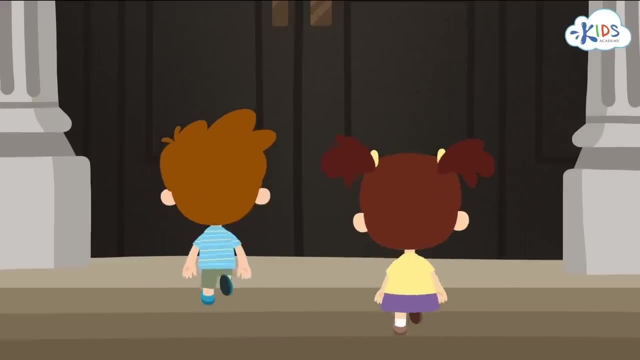 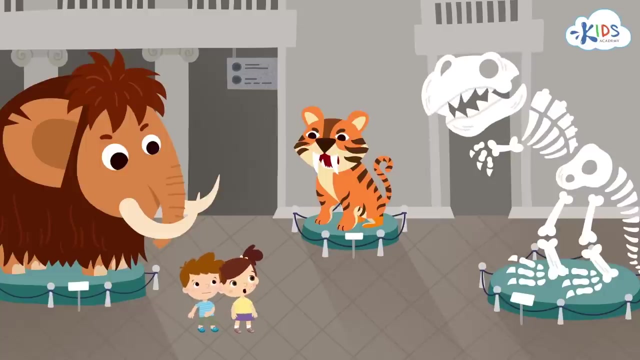 Where should we go now to have some fun? We can go to the National Zoo To see animals and birds from around the world, Or we can visit the National Museum of Natural History To see prehistoric animals like dinosaurs and saber-toothed tigers. 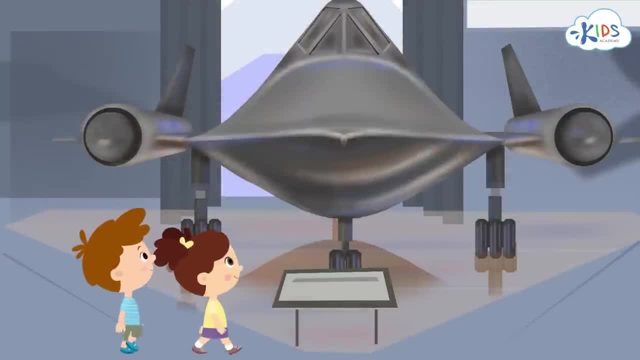 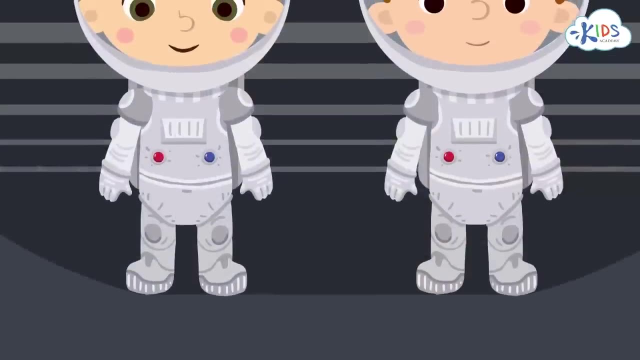 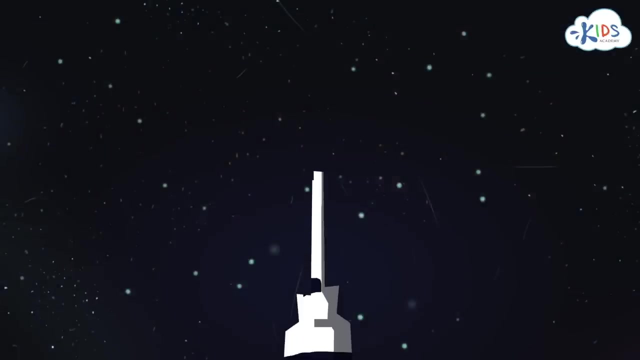 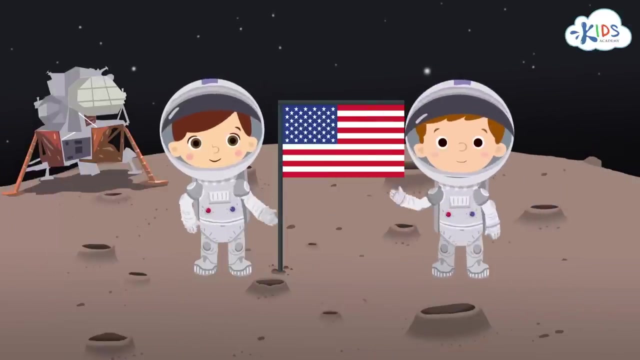 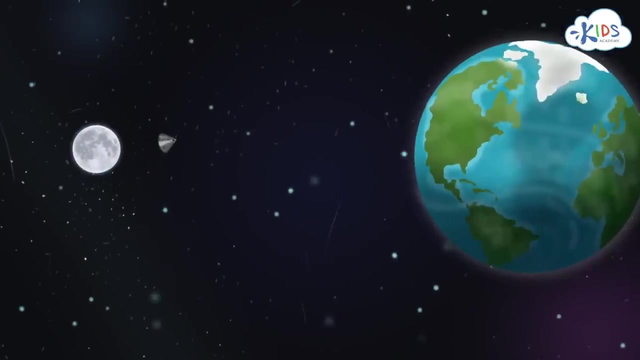 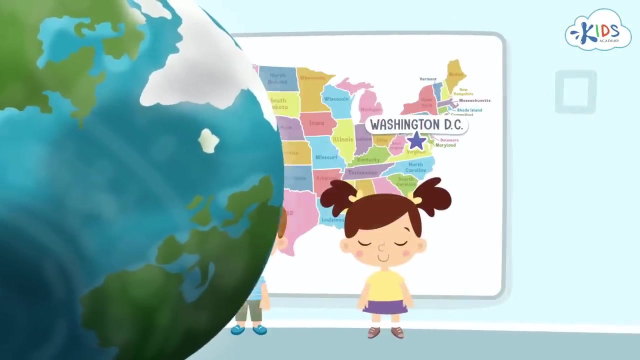 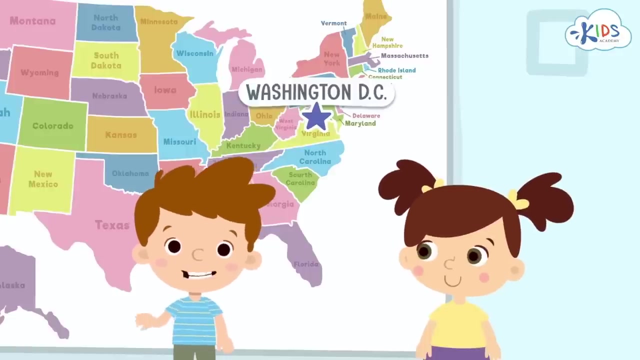 We could even visit the National Air and Space Museum to see airplanes, rockets and spaceships that reach the moon. Wow, This is so much fun. Washington DC is a very interesting city. We have visited lots of places, but there is still so much to see. 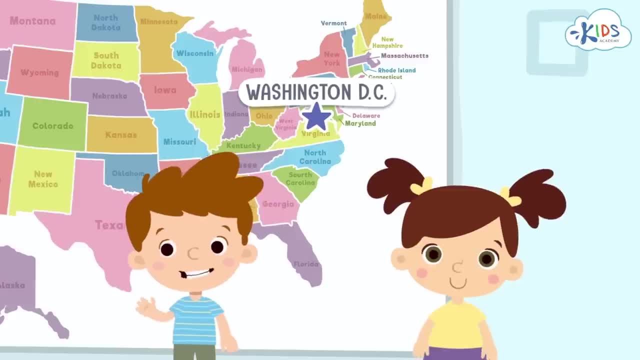 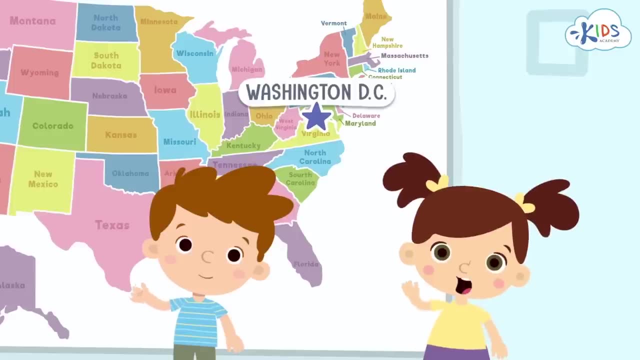 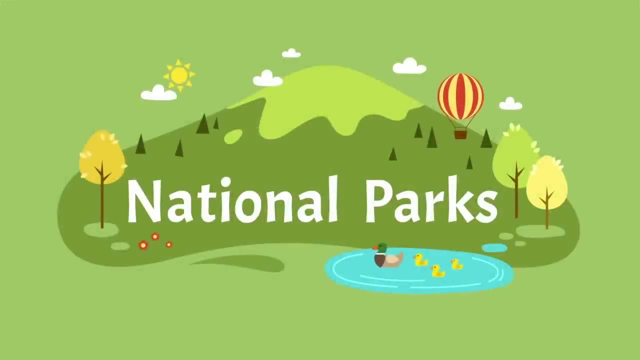 We will definitely come back again. What did you like best in Washington DC? What landmarks would you like to see? Thanks for watching. Goodbye, Hello. Let's get started on the lesson. Parks are an important part of the community. 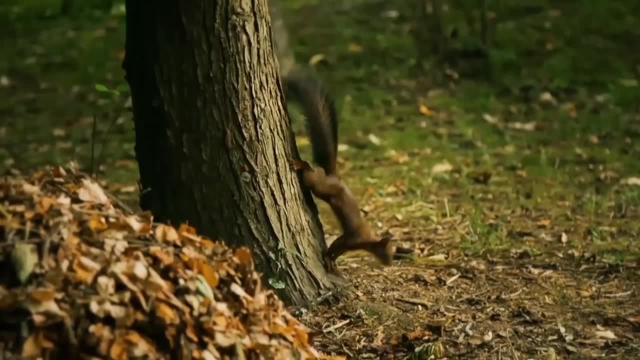 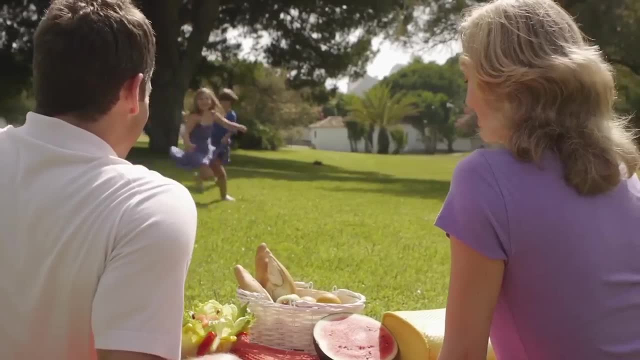 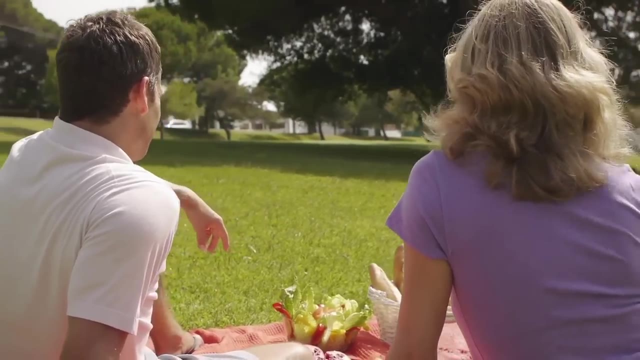 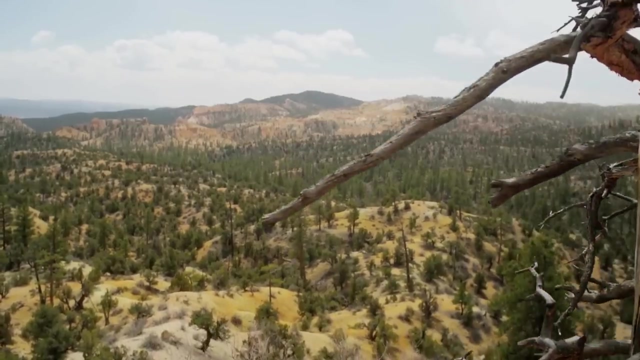 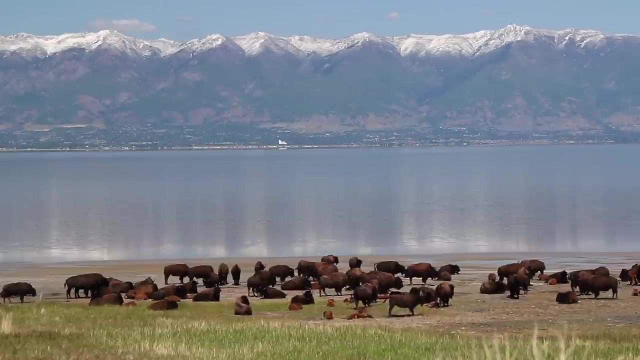 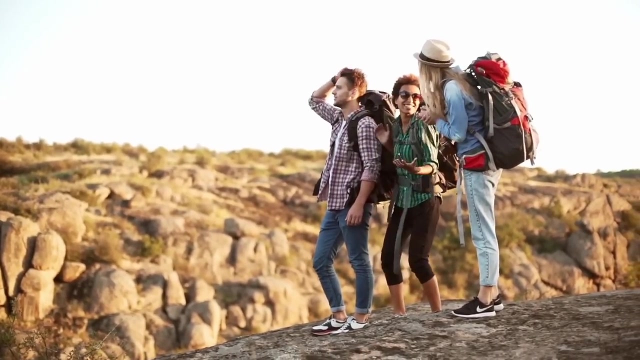 They are homes for many trees and animals. People like to visit community parks to relax, play or have a picnic. A national park is much bigger than a community park. It has many natural wonders for people to see. People from all over the world come to visit national parks. 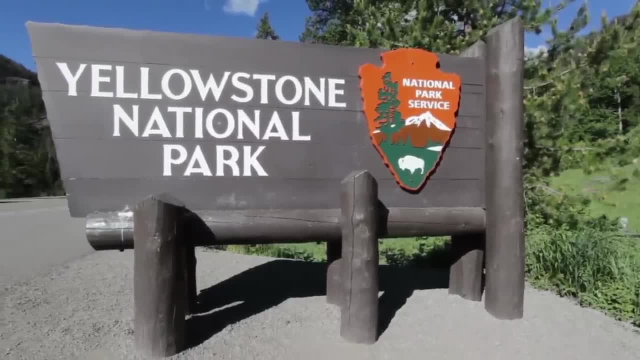 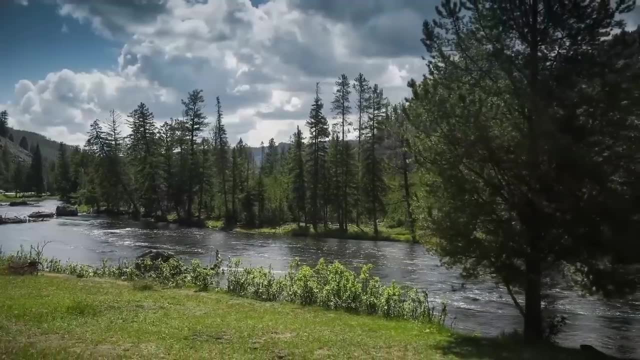 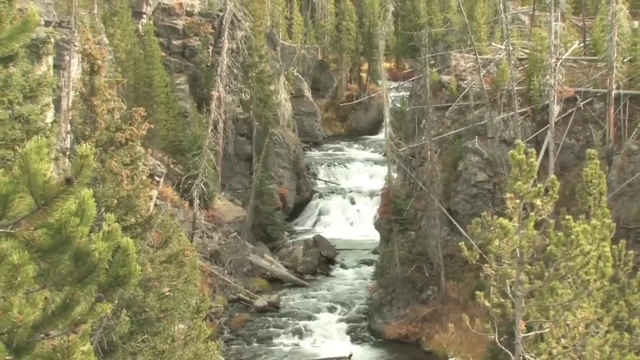 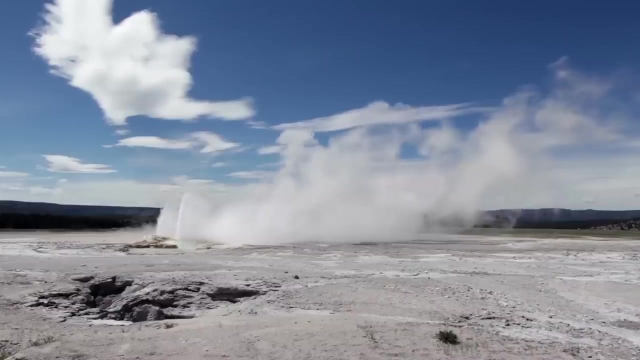 Yellowstone is the world's first national park. The park is large. It's located in three different states at once: Wyoming, Montana and Idaho. Yellowstone National Park is known for its geysers and hot springs, or fountains of hot water and steam.